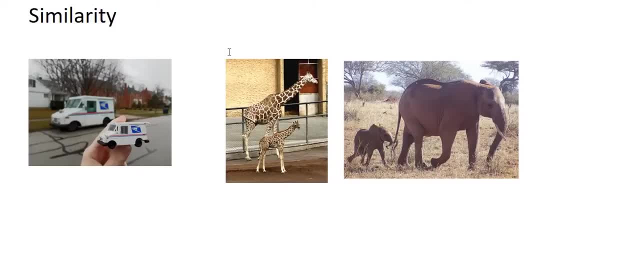 In this lesson we will talk about similarity. So from these three pictures I'm sure you can start to get an idea of what similarity is. So in the first picture we can see that there's a large postal delivery van, and then there's a smaller scale model of the delivery van. Here we can see. 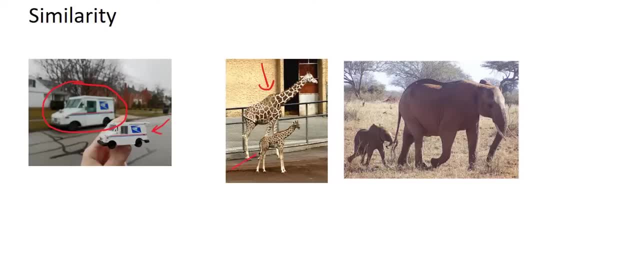 an adult giraffe and next to it is a baby giraffe, and then the same with the elephants. So similarity means that they don't have to be or they're not the same size, but they look similar. So all of their proportions and all of their ratios have to be the same. For example, it wouldn't make sense if 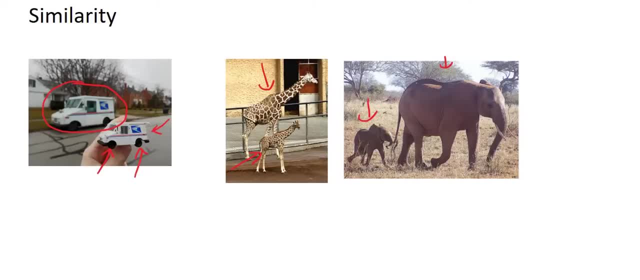 we take these wheels over here and we make them a lot bigger, because then it wouldn't look similar to the previous one. So the proportions have to be the same. So okay, but I'm going to explain this as we go along. Whereas in the previous lesson we looked at 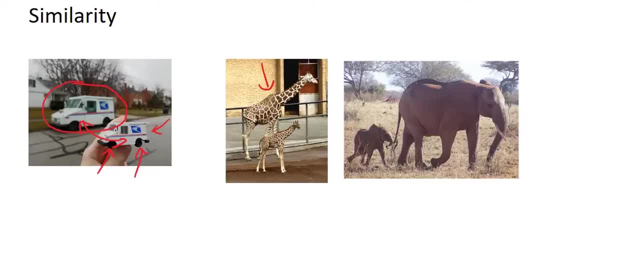 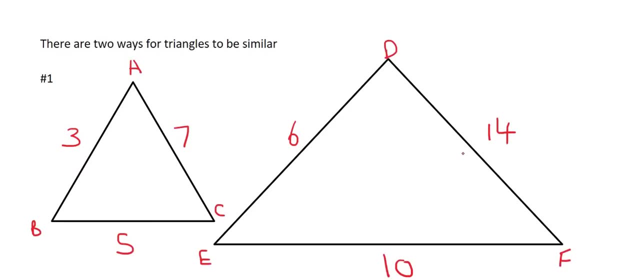 comparability. and then we looked at similarity. So the proportions have to be the same, So okay, but congruency? and that's when they looked exactly the same, Whereas similarity- they just look similar. Okay, now there are two different ways to prove that two triangles are similar, So don't confuse. 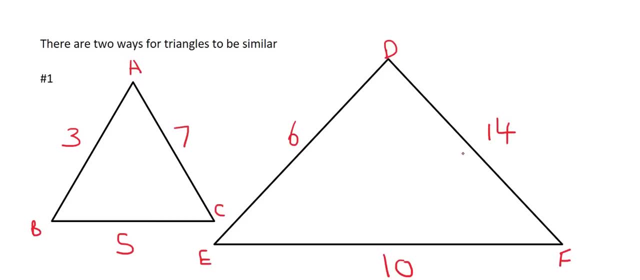 this with congruency, which we looked at in the previous lesson, where there are four different ways. In similarity, there are only two ways. The first one is the following Is to look. what you have to do is you have to look at the proportions or the ratios of the sides. So for 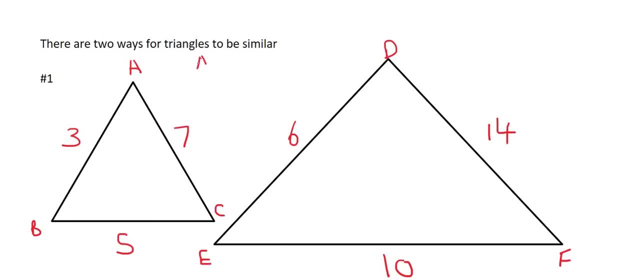 example, if you look at ab and you divide it by de, you would get 3 out of 6, which is the same as 1 out of 2.. If you then had to look at ac over df, you would get 7 over 14, which is the same as 1 over 2.. 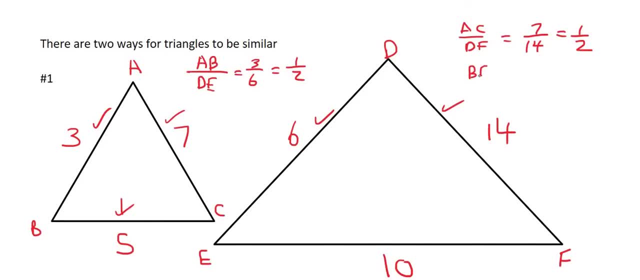 And then the last one is the proportion. So if you look at the proportions or the ratios of the sides, you would get 5 over 10, which is the same as 1 over 2.. So because we're getting that same ratio number, it means that these two triangles are similar. Later on in the lesson I'll show 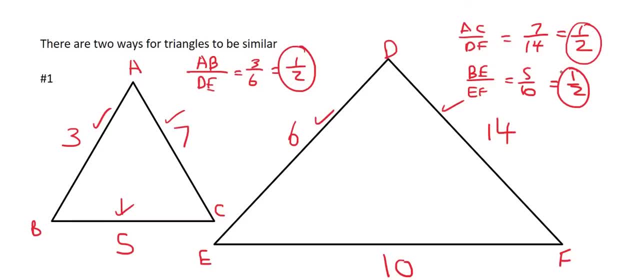 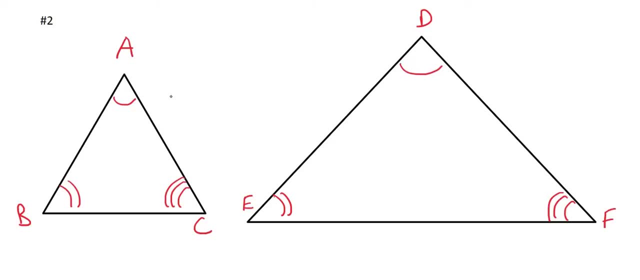 you exactly how to do it in the exam, but this is just an introduction. The next method is angles. If all the angles are the same, then the two triangles are similar. So if you look at the angles- So for example, if a is equal to d and b is equal to e and c is equal to f, then because of 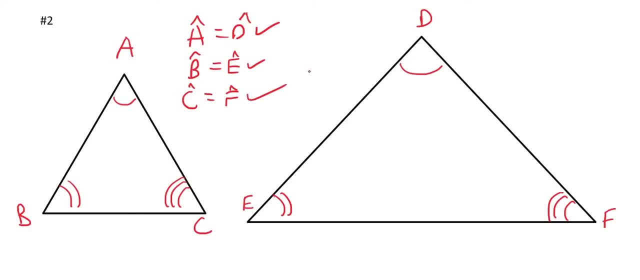 this, we can say that the two triangles are similar. Guys, that is the only way to prove that two triangles are similar, Either using the sides and their proportions, or using the angles. We're not going to use techniques like s and y. We're going to use the angles. We're not going to use the. 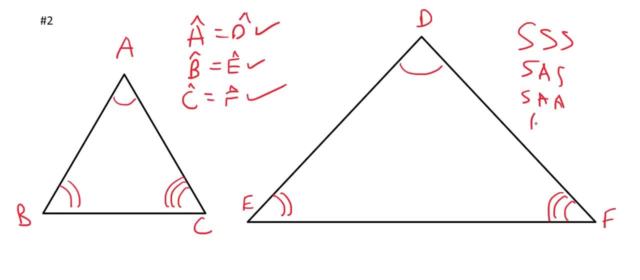 angles. We're going to use the angles. We're going to use the angles. We're going to use the angles ss and sas and saa and rhs. That is congruency. That is a totally different chapter. Okay, so let's. 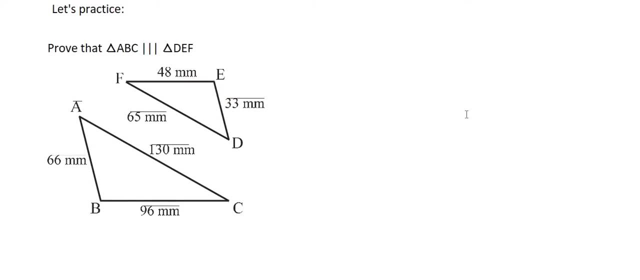 practice this. How would we do it in a test? Well, first of all, look how they ask the question. They say: prove that abc. Now look how they have three lines over here. So congruency had three lines going this way. Similarity has three lines going this way. Kevin, how am I going to remember this? 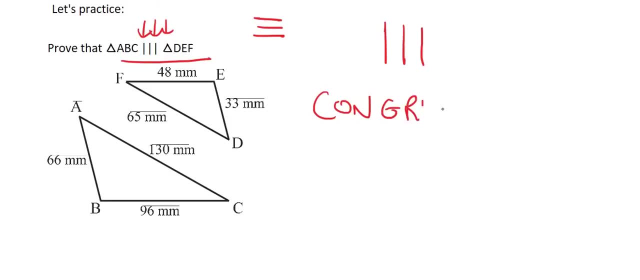 All right. well, we said that congruency had three lines going this way. So congruency had three lines going this way. So congruency, you should write it out in capital letters or congruent, and you would see the e over there to show you the three lines. Can you see the e? Then similarity: you can also. 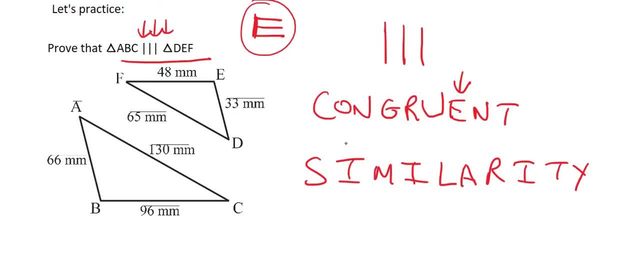 use that technique. Check this out: If you write out the word similarity, check what you get: There's an i, There's an i and there's an i, And so those are the three i's that are next to each other. We. 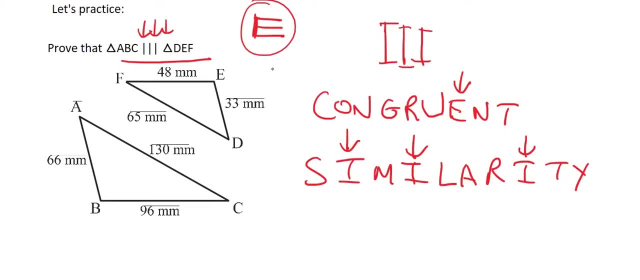 can see it over here, And so with that, you will never forget which one is similarity and which one is congruency. Now I want us to prove that these two triangles are similar. Now we said that there's only two ways to do this: Either using sides or angles. Clearly, we have to use sides over here. So how? 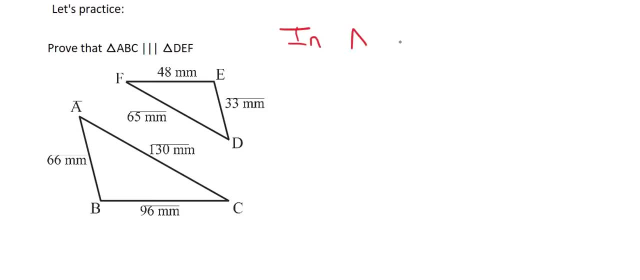 would we do this? in an exam Like this? You would say: in triangle, just like we did with congruency. you would just use their one, So abc, and in triangle, def. So you just tell the teacher which triangles you're going to work in. Now we need to look at the sides So we could, for example, say: 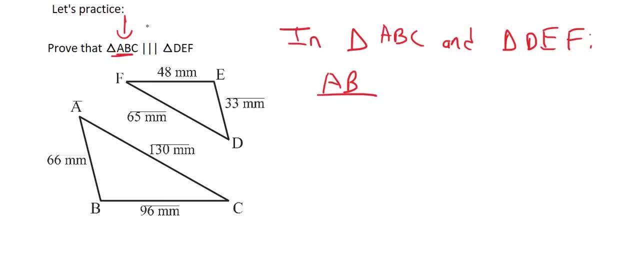 that abc is a triangle. So we could say that abc is a triangle. So we could say that abc is a triangle. So if we look at the sides, we can say that AB goes with DE. If you're struggling to see which one goes with which, just look at the order of the letters. So AB will go with DE, So we can say AB. 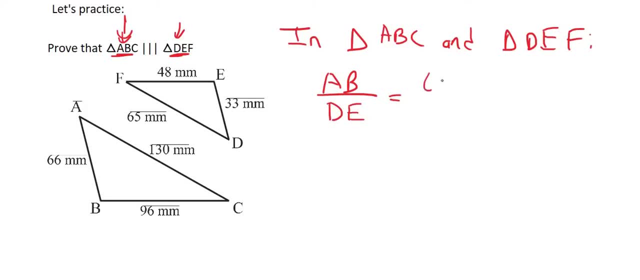 over DE is equal to 66 over DE, which is 33.. And if you simplify that you're going to get 2.. Then we can say: now we can look at another two letters. So for example, we could look at BC and EF. So we could say BC over EF. 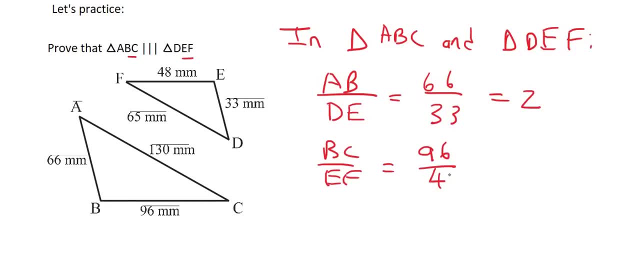 and that would be equal to 96 over 48, which is also equal to 2.. Then we could look at another two sides, which would be the first one and the last one. So that would be AC over DF and that would be 130 over 65, and that is also equal to 2.. So, because all three of them are giving us a 2, 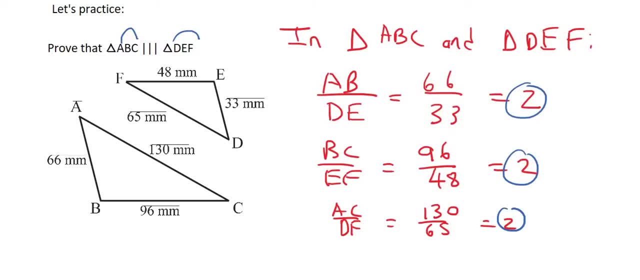 we can say that these two triangles are similar, But what would our reason be? Well, you would first say: therefore, triangle ABC is similar to triangle DEF. Why? Because the corresponding sides are in proportion. So you say: corresponding like that, sides are in proportion like that. So here's the 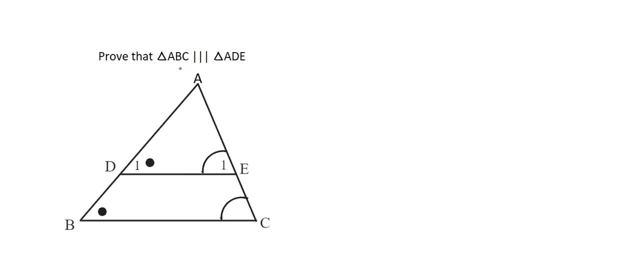 next one and this one. they want us to prove that triangle ABC is the same as or similar to triangle ADE. So clearly we need to use angles for this one, because all we can see is angles. They haven't given us any sides. So if you're stuck and you don't know where to go or where to start, 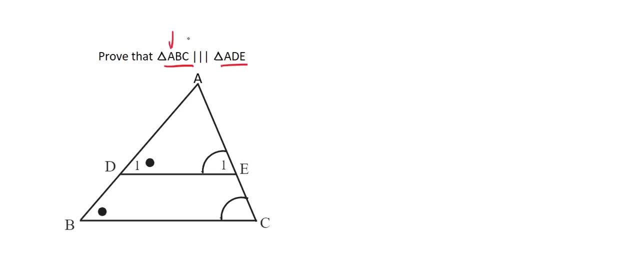 always look at the order that they've given you. So why would A be the same as A? So why would these two be the same? Well, I mean, if I had to pull these two triangles apart, it would look like this: You would have ADE, and then you would have. 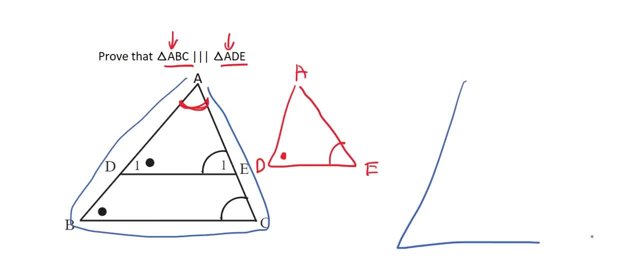 ADE a, b, c. so let me quickly draw that one. would you agree with me that they both use angle a, and so that will have to be the same for both of them, and so what this means is that we can. we should first tell the teachers which one we're working in, so in triangle a, b, c and triangle a d. 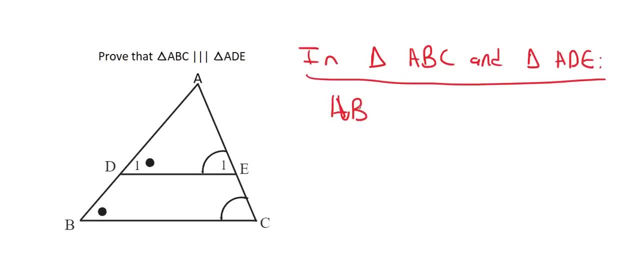 e. we can say that a b, sorry. we can say: angle a is equal to angle a. why? because it's common to both of them. then we can say that now you look at the next one, that's a b and the next one is a- d. why would b and d be the same? well, they've given us that, so we could say angle b is equal to angle. 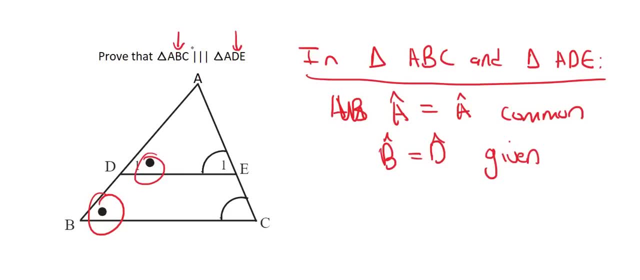 d, because they gave us that that's given. and then we look at the next one, c and e. so angle c would equal to angle e, and that's also given. oh, but we should call it e1, can you see that? because they they've called it e1 specifically, and so therefore we've got. 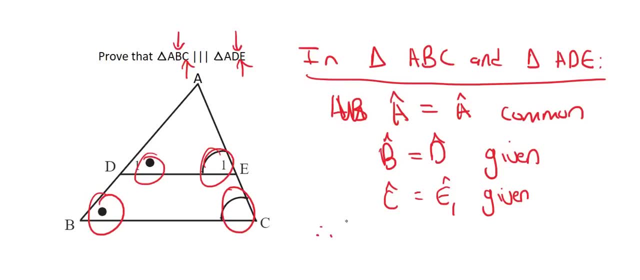 Oh, those three angles being the same, and so we can say: therefore, triangle abc is similar to triangle ade. but now we're not going to say corresponding sides are in proportion, because here we're using angles, so we just say a, a, a, or you don't have to put the commas there, so a, a. think about that in. 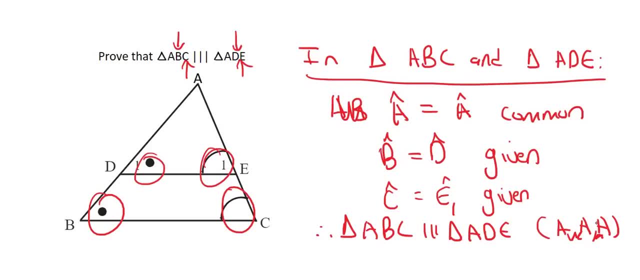 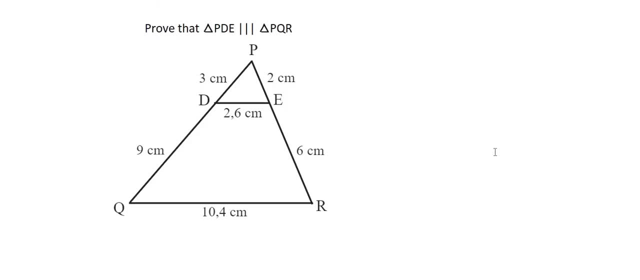 congruency, we would say something like side side, side side, angle, side, but when you're using similarity with angles, you just say angle, angle, angle, and so the last question for this lesson is the following: prove that triangle pde- so this is the small one here in red- is similar to pqr, pqr. 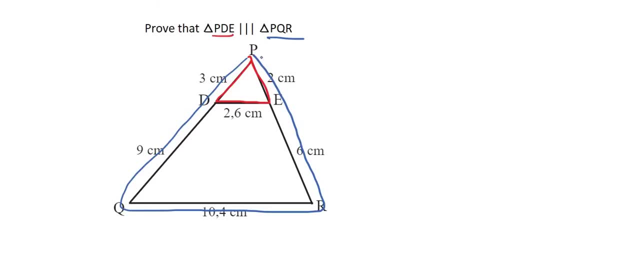 now, guys, remember there are only two ways to do similarity: either using angles or sides. clearly, this one is going to use sides. so we start off by saying, in triangle p, d, e and triangle pqr, and now we need to use sides. now my hint would always be to just use the letters. 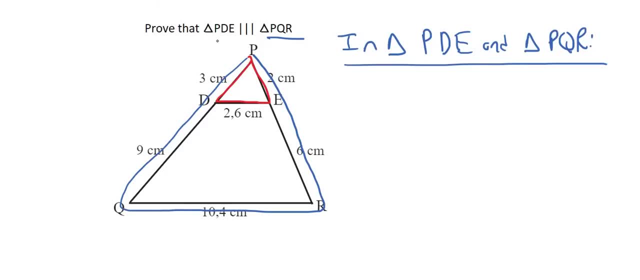 that they give you. so because we're using sides, now you're gonna. you can't just say p, that would be an angle. so you're going to look at pd. so let's look at pd. now, what does that go with in the other triangle? well, that goes with pq. so let's say pd over pq and let's fill in the value. so pd is three. 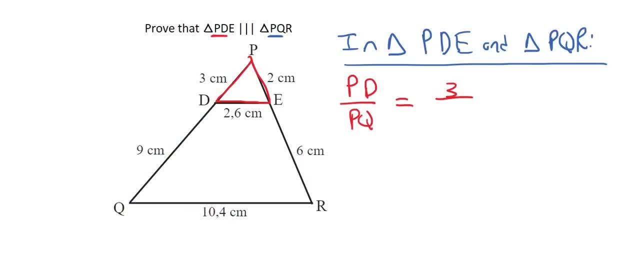 is not 9.. Be careful for that, guys. A lot of people fill in a 9 over here, but PQ is the 3 plus the 9, and so that's going to be 12.. And if you work that out on your calculator, that'll be.